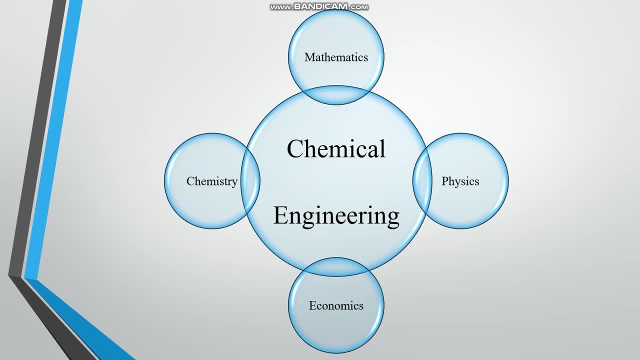 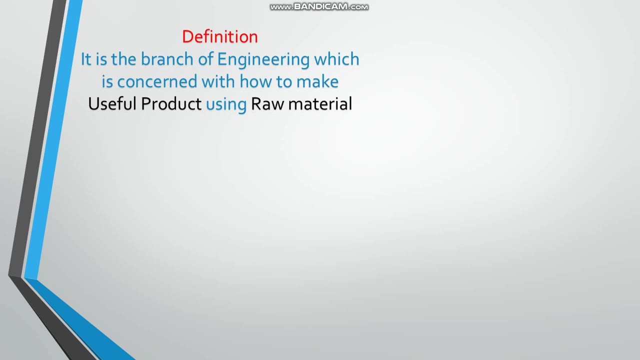 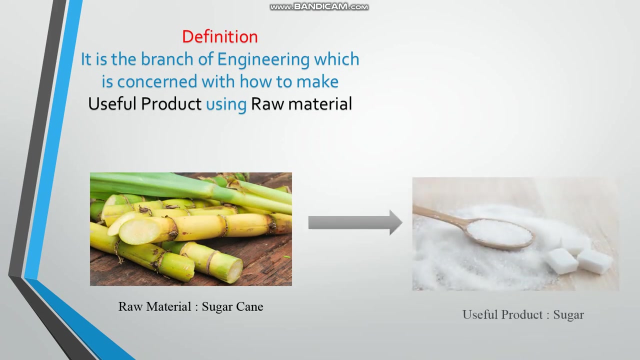 it involves physics laws in observing fluid flow, laws of chemistry. in the subject of physics engineering, it can be defined as the branch of engineering in which we study the conversion of raw materials into products. for example, in sugar industry, sugarcane is our raw material, which is converted into sugar, which is the final. 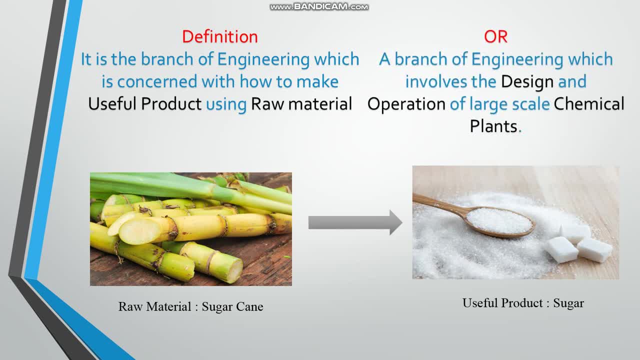 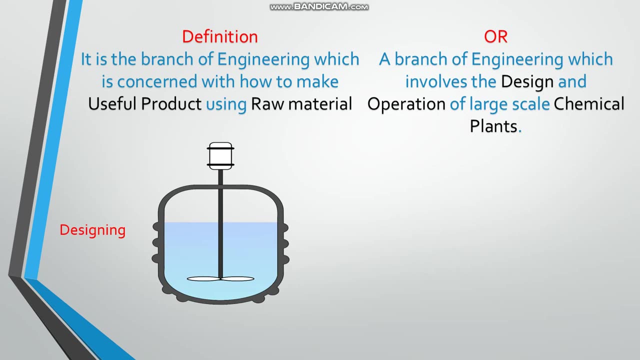 useful product. it can also be defined as the study of design and operation of large-scale chemical plants. what is meant by design and operation? let's say we have a batch reactor which is our core equipment of chemical engineering. designing is basically finding height, diameter, power and other parameters like 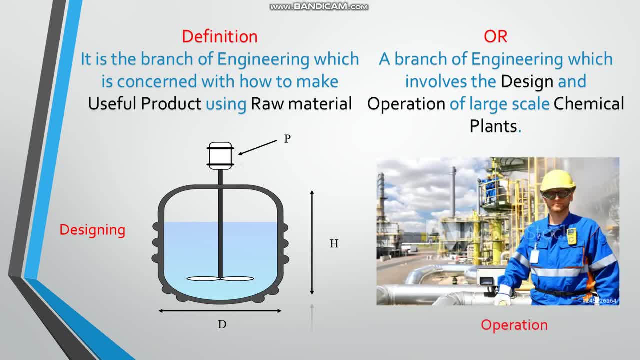 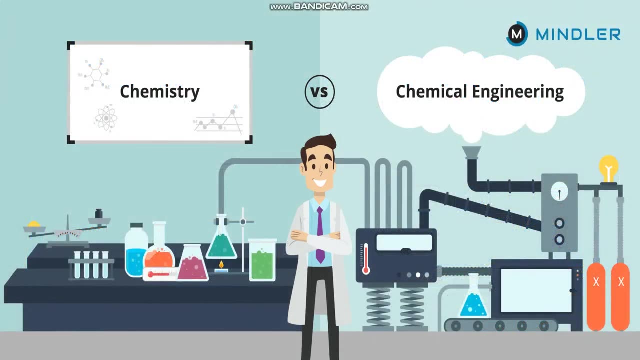 this in operation. we generally look after chemical plants. we check either flow rates, concentration and other parameters are according to our requirements or not. many of us confuse chemical engineering with chemistry and choose chemical engineering because they like chemistry. but I want to tell you it's not like that. there is a huge difference between chemistry and chemical. 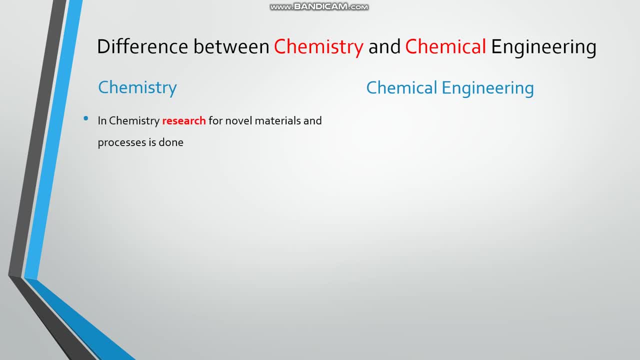 engineering in chemistry research for new chemicals, their method of preparations. on the other side, chemical engineers use this research in designing and produce these chemicals on large scale. those who study chemistry are recognized as chemists and for chemical engineering recognition is chemical engineer. chemists work in laboratory and chemical engineer work at chemical. 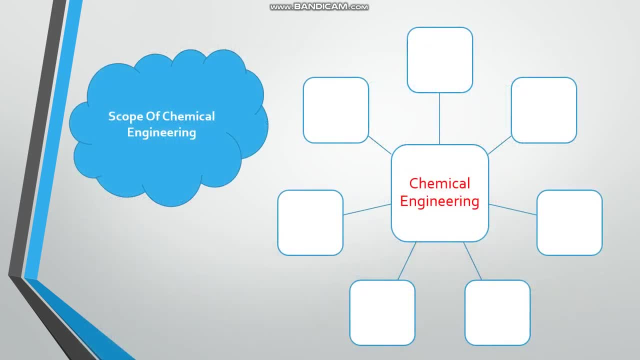 plants. chemical engineering is also called universal engineering due to its large applicability. I have listed some of sectors which are covered by chemical engineering, for example, food and drinks, energy sectors- including oil, gas and nuclear plants, information technology, education, chemicals and allied products, fertilizers, plastic and metal industry. it is very important to know the role of a